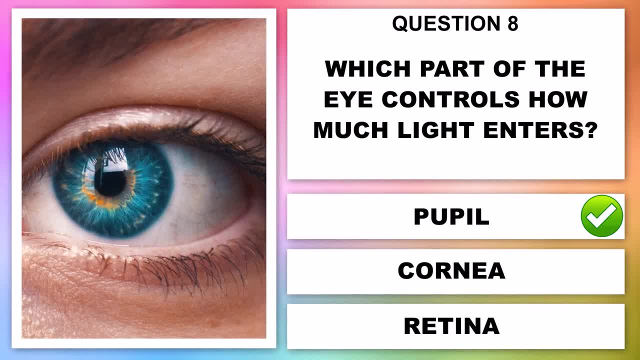 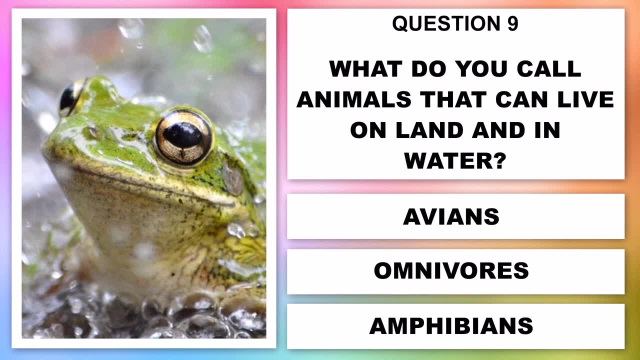 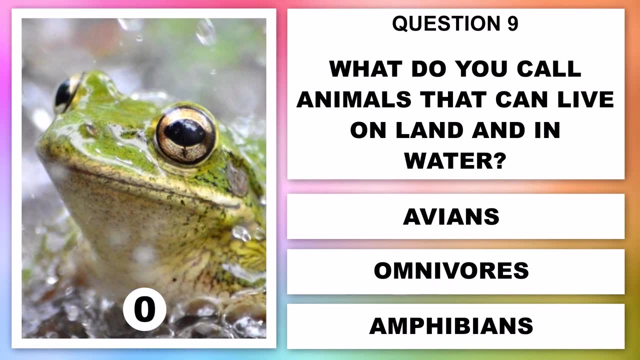 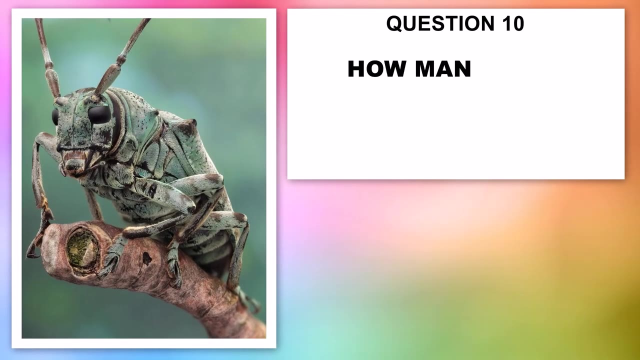 The pupil: Question 9.. What do you call animals that can live on land and in water- Avians, omnivores or amphibians? Amphibians- Question 10. How many legs do insects have? Amphibians- Question 11. How many legs do insects have? 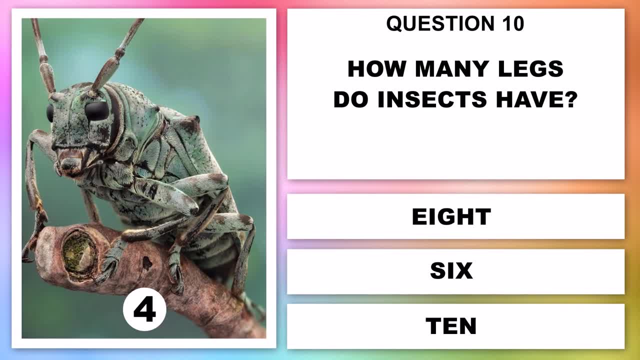 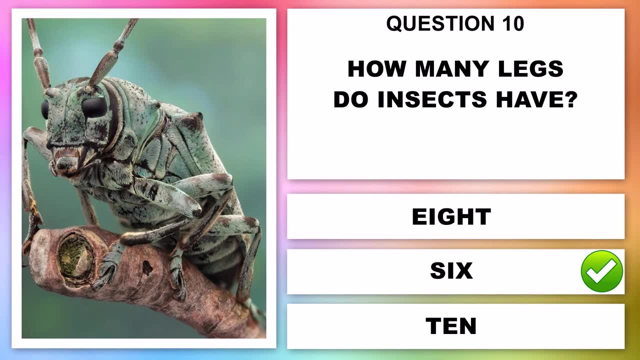 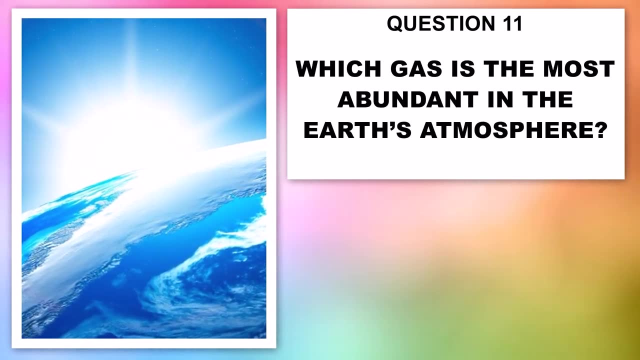 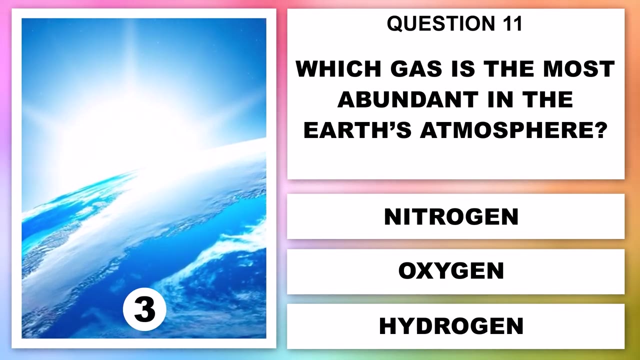 Eight, six or ten. Eight, six or ten Six. Question 12.. Which gas is the most abundant in the earth's atmosphere? Which gas is the most abundant in the earth's atmosphere? Nitrogen, Oxygen or Hydrogen Nitrogen? 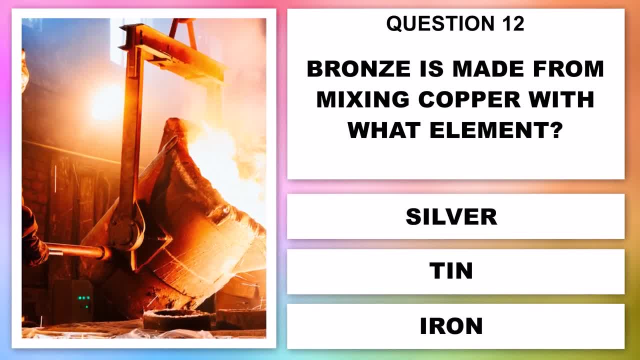 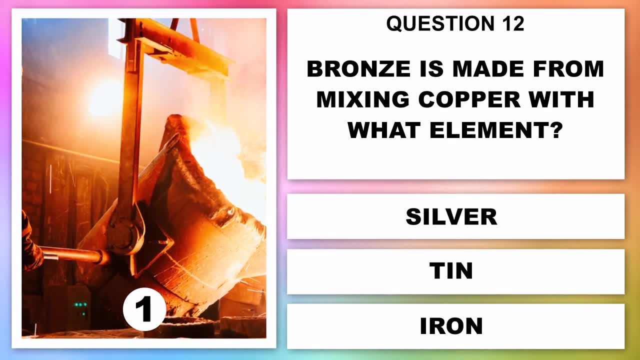 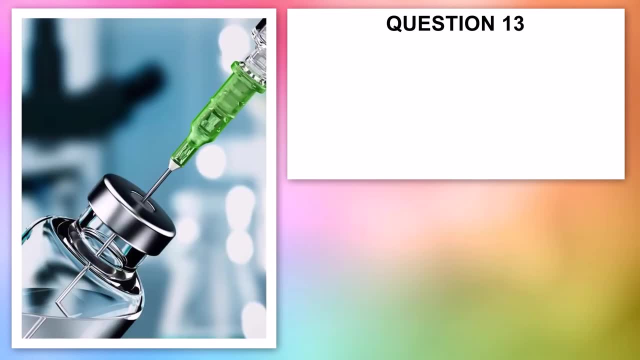 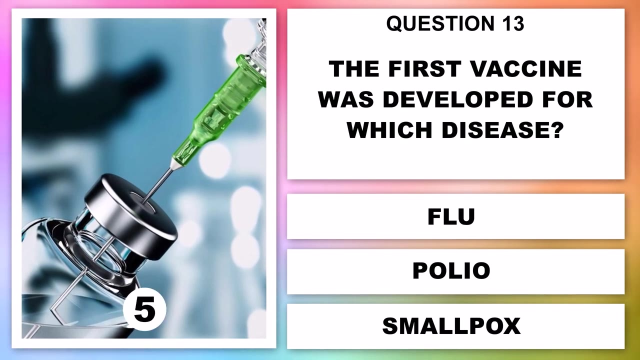 Question 13. Bronze is made from mixing copper. with what element? Silver, Tin or Iron Silver? Question 14. The first vaccine was developed? for which disease? Flu, Polio or Smallpox? Flu, Polio or Smallpox. 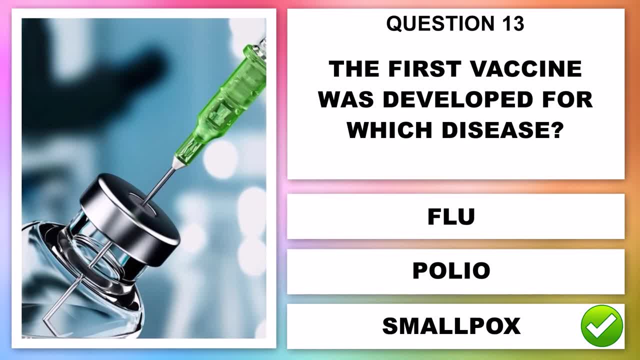 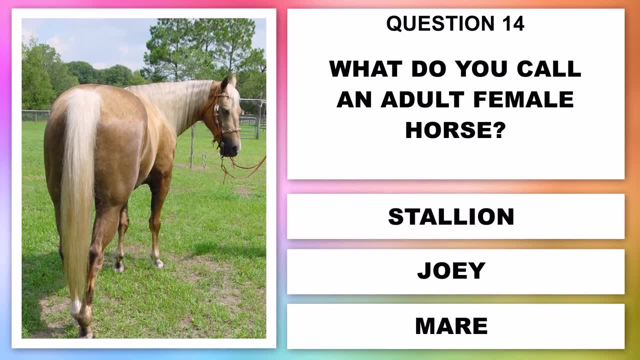 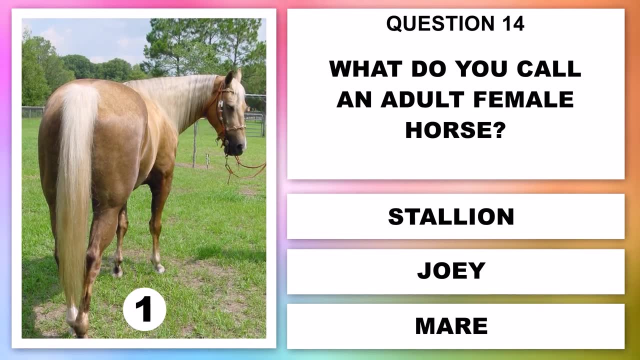 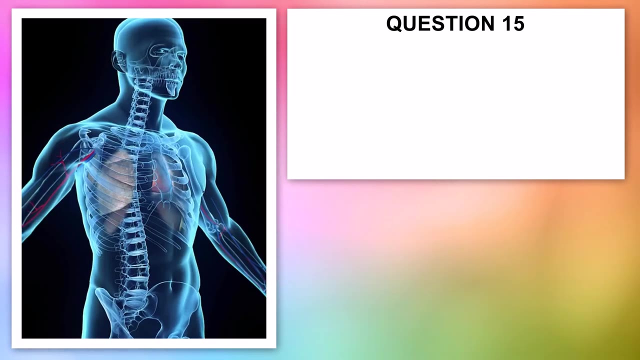 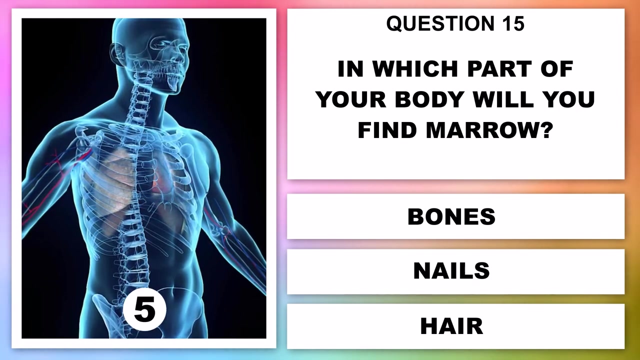 Smallpox, Question 15.. What do you call an adult female horse? A stallion, a joey or a mare? A stallion, a joey or a mare, A mare? Question 16. In which part of your body will you find marrow? In the bones, the nails or in the hair? 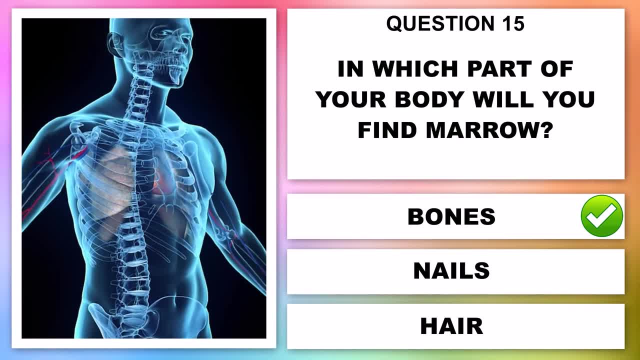 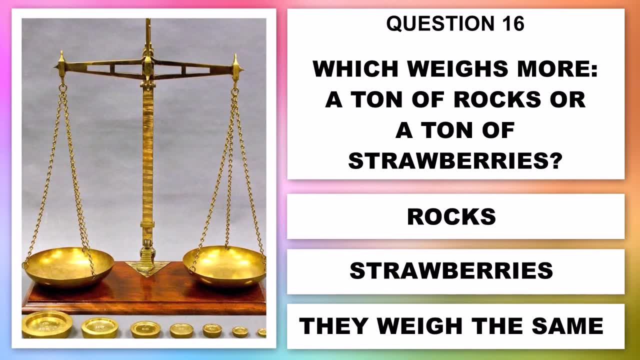 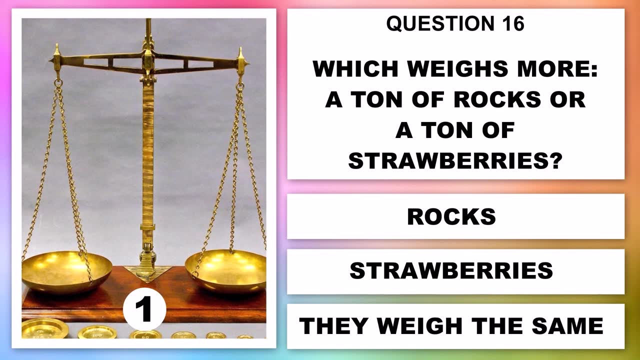 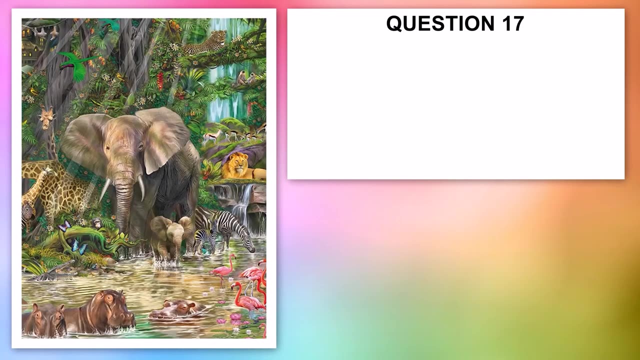 In the bones? Question 17.. Which weighs more, one ton of rocks or one ton of strawberries? The rocks, strawberries, or do they weigh the same? They weigh the same. Question 18.. Which one of these is a mammal?